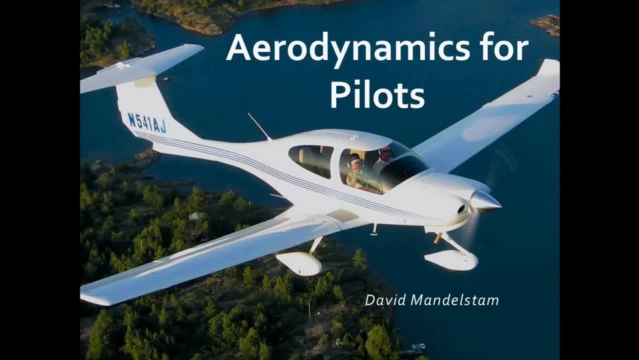 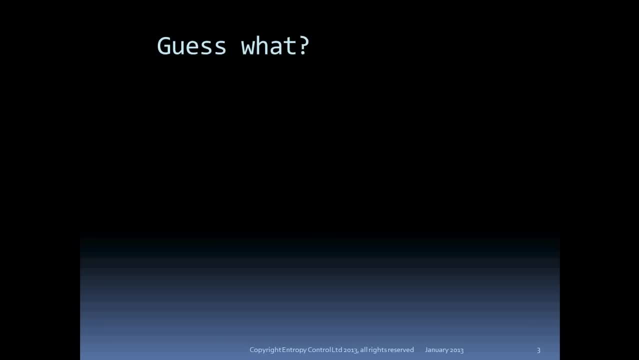 Hello again and welcome to the fourth lecture in this series. This is a lecture on stability and control. Stability is the tendency of an aircraft to return to its original attitude after a disturbance. Now, contrary to popular myth, aircraft are generally not completely stable. nor do they have to be. 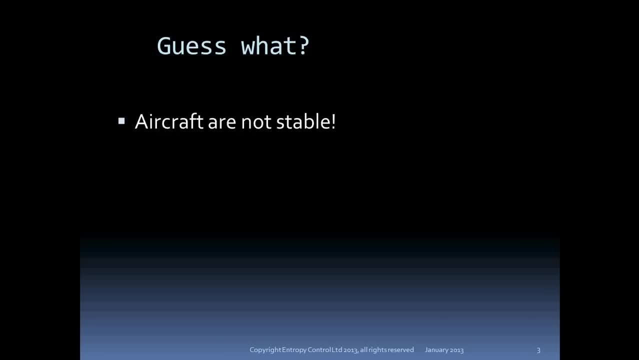 It's enough that the motions are slow enough for a pilot to be able to handle them. There are trade-offs. For instance, if an aircraft is too stable in side-slip, it will suffer from a sickening motion called Dutch Roll. Aircraft can be made stable, For instance. free-flight model aircraft are usually quite stable. 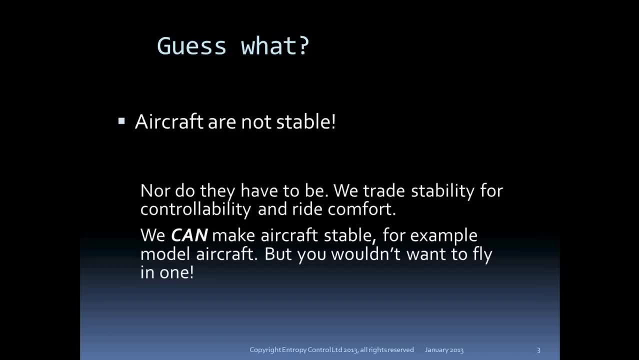 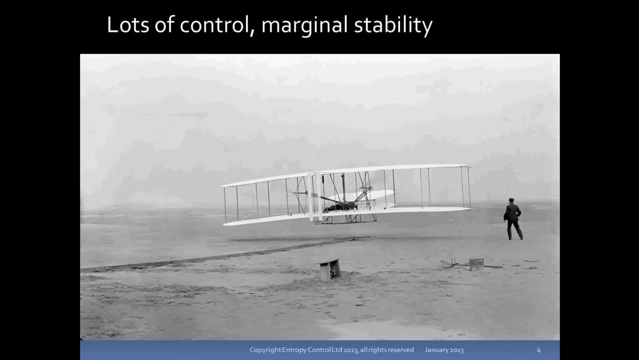 But for passenger aircraft we normally have to live with some instability in return for comfort. To go back to the very beginning of things, the Wrights created Aircraft that were very responsive to the pilot but had little stability. Note the an-an-hedral, that's the negative dihedral on the original Wright flyer. 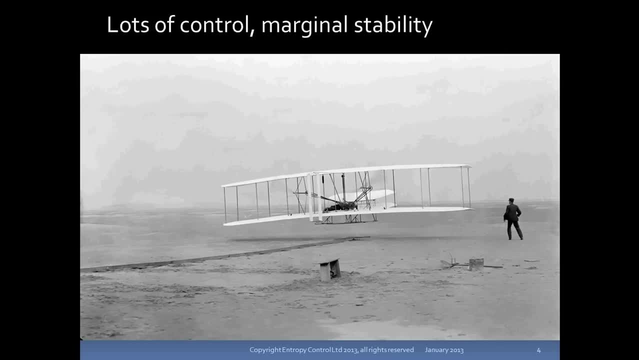 One would have to be quite vigilant in keeping the wings level, as there would have been no side-slip stability at all. Reportedly, longitudinal stability was also pretty much neutral. These machines were a real handful to fly, but the pilot did feel totally in control. 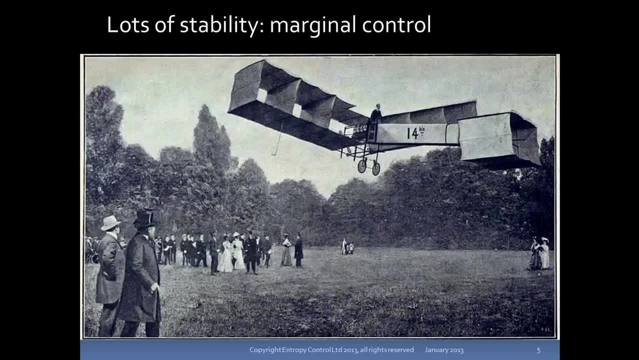 In contrast, here we have Santos Dumont's 14bis. This was an ultra-stable aircraft. Directional control must have been quite poor. For instance, it looks like there's no roll control at all. The pilot had some longitudinal control, but he was really just more of a passenger. 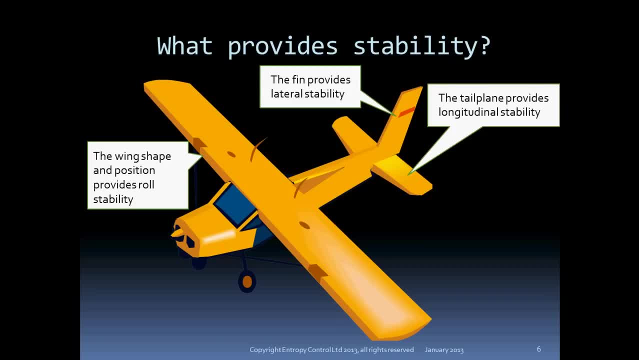 So what provides stability to the aircraft? The most straightforward component of stability is the fin. We've seen this in the previous video. Notice how it's held by one pin, which provides stability in yaw. The fin acts much as the feathers do on an arrow. 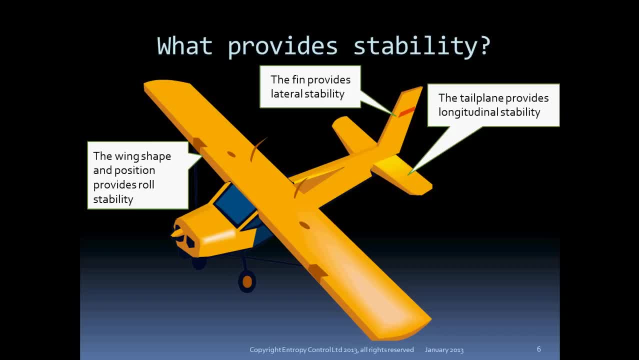 As long as the CG is well forward of the central lateral pressure, the aircraft will be stable in yaw and will fly straight. The tailplane looks as if it is much the same as the fin, but in fact its behaviour is more complicated. In normal flight the fin carries no loads. 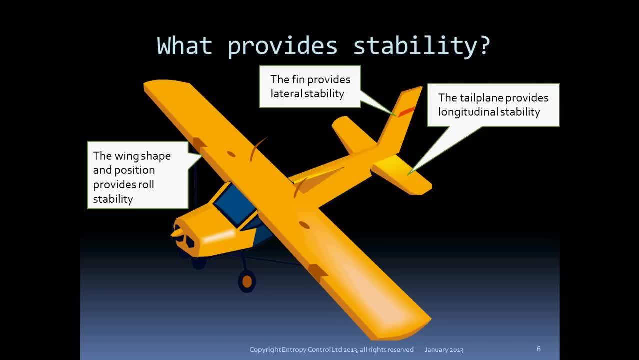 carry aerodynamics in all phases of flight, so its effect is heavily dependent on the position of the central gravity. The tailplane can be behind the main wing or in front of the main wing, in the so-called canard configuration, but the rules of stability dictate that the 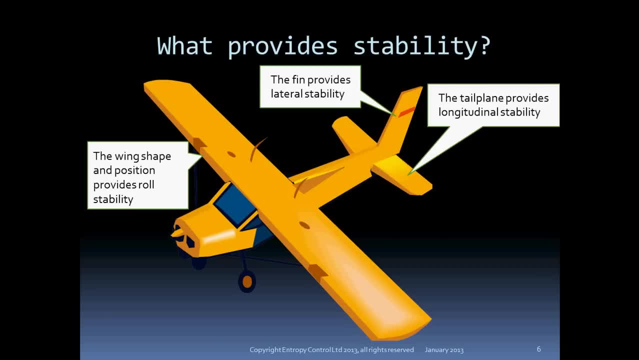 front wing has to be at a higher angle of attack than the rear wing. It's not very efficient to have a small wing in front working very hard with a big wing behind just loafing along. so canards tend to be much larger than normal trailing tailplanes, In fact. 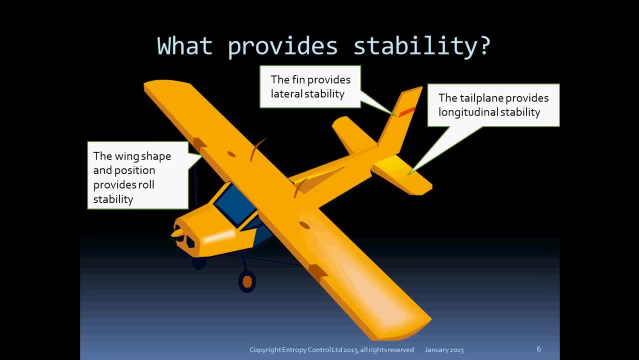 as the designs are optimized, canards tend to grow and the main wing tends to shrink until the aircraft begins to look much more like a normal conventional aircraft. Also, note that the loads on a normal trailing tailplane do not always have to be down as 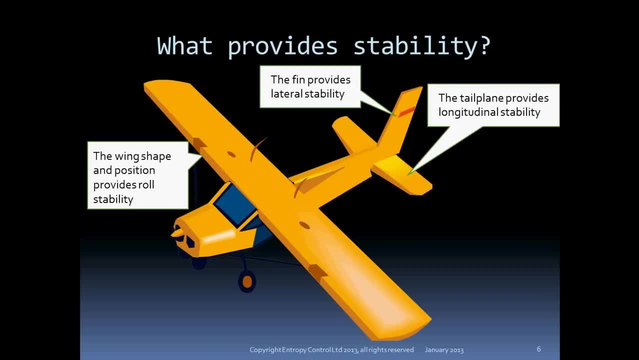 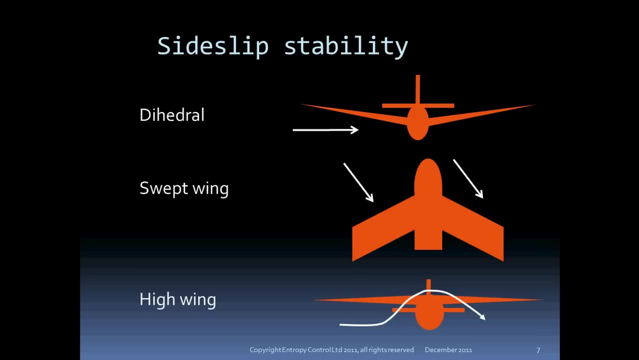 is the conventional wisdom. It's possible to load and trim an aircraft such that both surfaces are providing positive lift. Stability in side-slip has more than one component. Typically, side-slip stability is provided by a dihedral. A side-slip creates an airflow that causes the upwind wing to 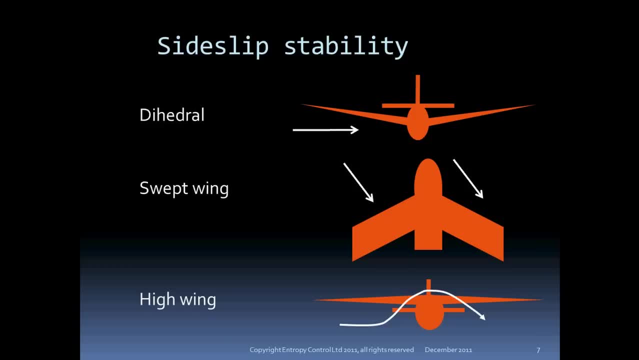 be at a higher incidence than the downwind wing, rolling the aircraft out of the slip. Similarly, a swept-wing aircraft has the upwind leading edge more at right angles of the flow than the downwind wing, also providing a greater incidence of the downwind wing. This is because 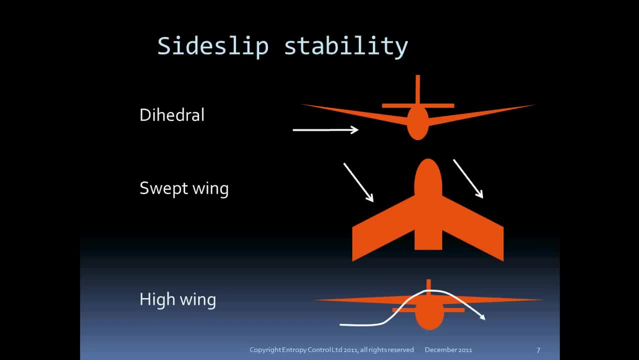 the upwind wing is more at right angles of the flow than the downwind wing, also providing a greater incidence of the downwind wing. For a high-wing aircraft, the fuselage interference in a side-slip provides locally higher incidence on the upwind wing rolling the aircraft. 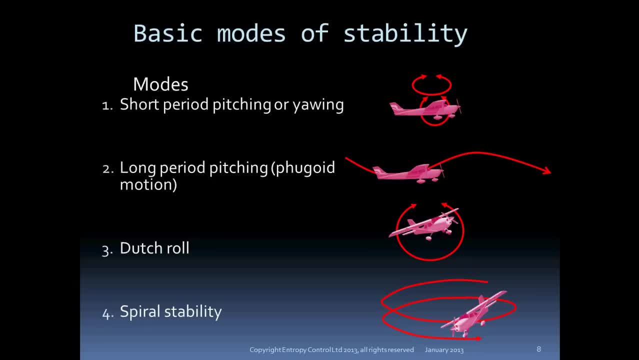 So now let's have a look at the modes of stability. You'll have heard of the term static and dynamic stability. Static stability is the tendency for the aircraft to return to its original state. So let's have a look at the modes of stability. 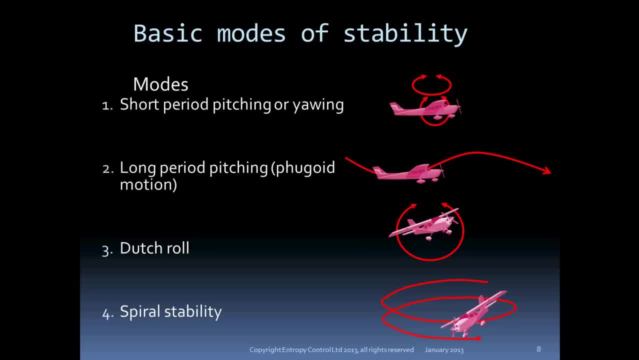 Static stability is the tendency for motion, or motion caused by a disturbance, to gradually dissipate. You cannot have dynamic stability unless the motion is statically stable. But static stability does not necessarily mean that the motion is dynamically stable. Actually, from a practical standpoint, these classifications are not very useful. 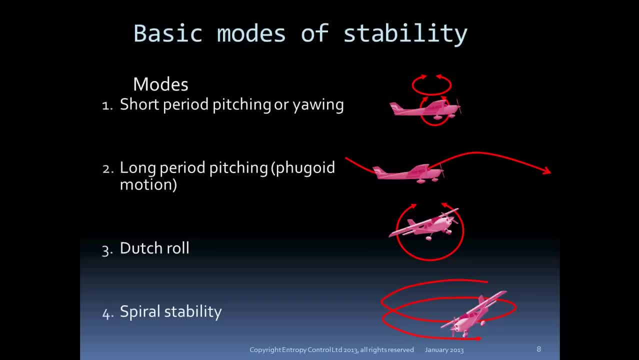 What matters more are the time scales, the motions. If the timescales are long enough, a pilot can cope even if there's some instability. Now, talking about the modes, the short period oscillation is what you get if you kick the. 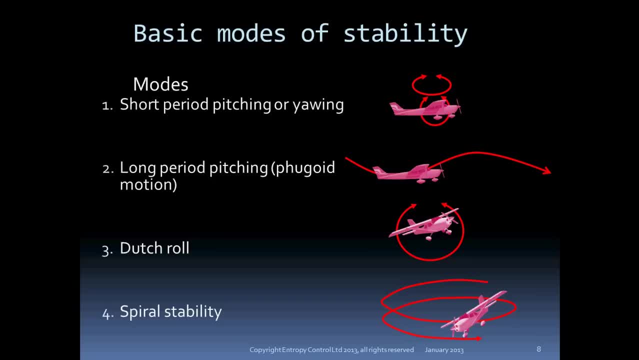 rudder or push the stick. The aircraft very rapidly returns to forward flight. The motion has a very short period and is very heavily damped. The second mode is a long period oscillation in speed and altitude called the fugoid. Then there is Dutch roll, a motion in yawn. 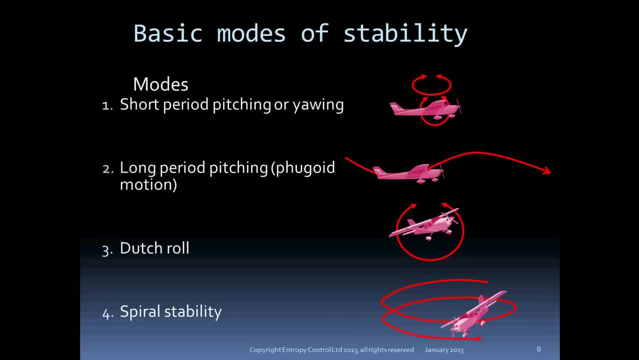 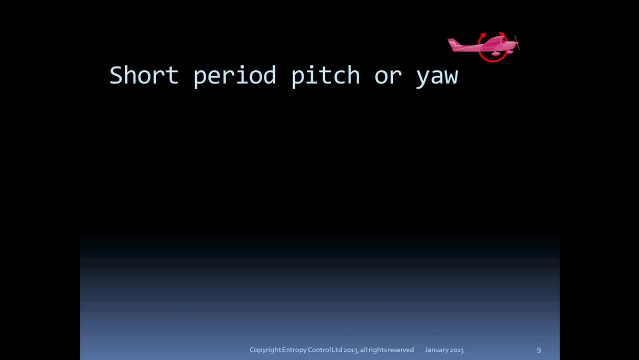 roll, named after the rolling gait of a skater. Finally, we have spiral stability, which is the ability to return to straight flight after dropping a wing. Now examining these modes of stability in detail, let's have a look at the short period. 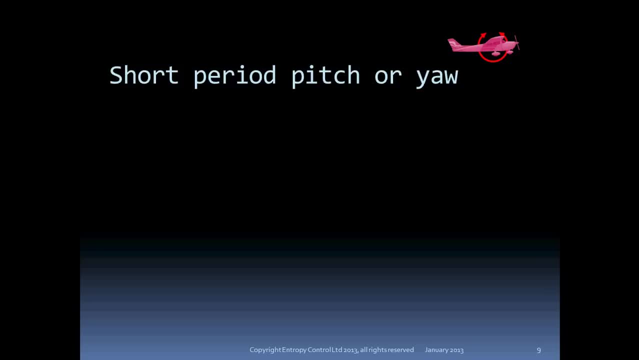 stability in pitch and yawn. If you disturb the flight in pitch or yawn, the aircraft rapidly returns to its flight path and the motion is heavily damped. This is a good thing, because the timescales involved in the movement are much too small to be dealt with by human reactions. 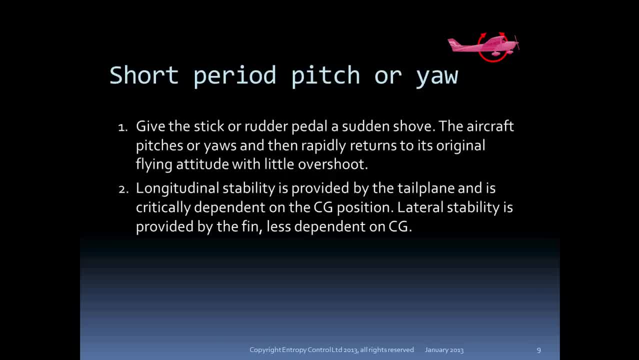 It is the center of gravity position that determines the short period stability in pitch. The aircraft has to be loaded inside the CG limits if it is to be at all controlled. Your stability also depends on CG position, but much less critically so. Modern fighters with on-board computers are able to operate with no short period stability. 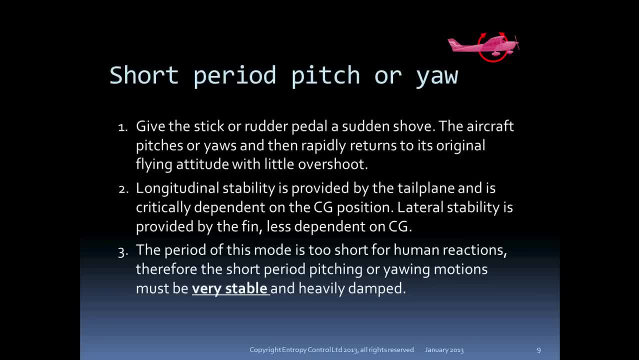 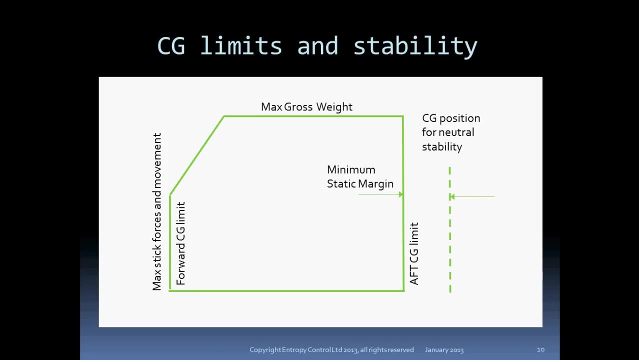 simply because the computer reactions are fast enough. You don't have that luxury, so you really need to watch your CG position. There is a center of gravity position where the aircraft is neutrally stable in short period motion. It is found in test flight by measuring stick forces and movements required to pull extra. 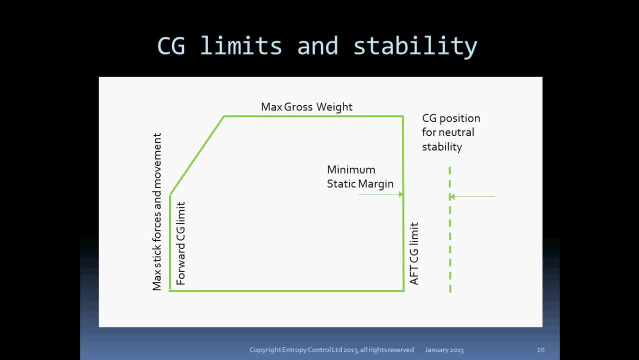 Gs at different center of gravity positions and then extrapolating the curve back to the CG position for neutral stability. There is also a center of gravity position where the aircraft is neutrally stable in the CG position and then extrapolating the curve back to the CG position for neutral stability. 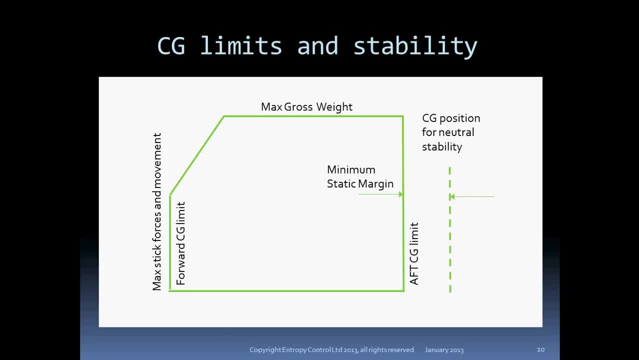 A margin of safety is defined as the static margin of safety, which defines the aft-most allowable center of gravity position. The forward CG limit is usually fixed by the ability to rotate the nose for take off and landing. As stick forces increase with gross weight, there is often that sloping portion to the 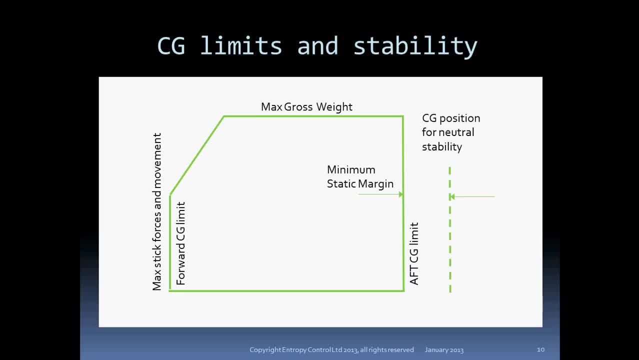 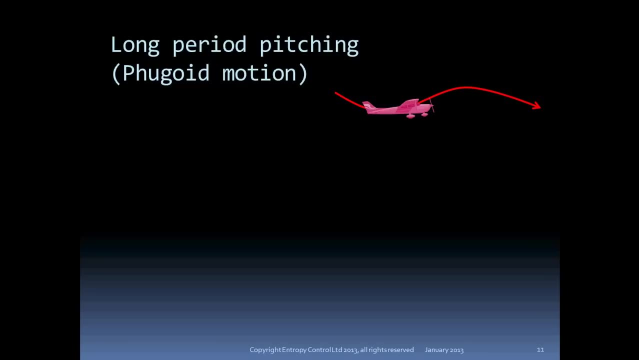 front of the CG limit. Finally, the top of the envelope is given by the maximum gross weight, which is a structural or performance limitation. So now let's have a look at the Fugoid. The Fugoid motion may or may not be stable. 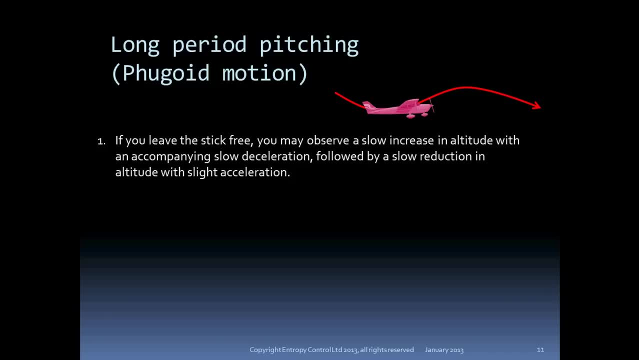 It involves a slow climb with decreasing speed, followed by a slow descent at increasing speed, and repeats ad infinitum. The period is about 30 seconds for a lighter aircraft. Even when the motion is stable or limiting, the pilots can generally cope without too much trouble. 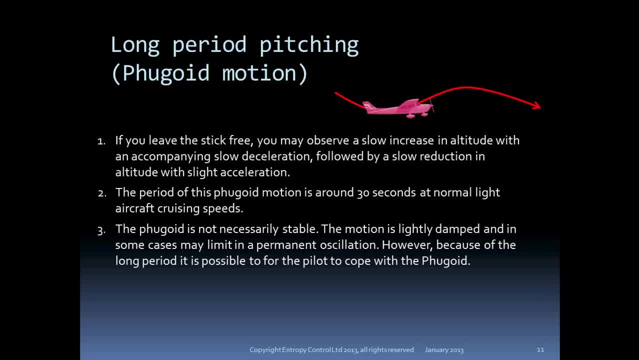 though maintaining altitude can be difficult. A Cirrus aircraft has a reputation for exhibiting a Fugoid under certain circumstances, and that makes maintaining altitude without the use of an autopilot a bit of a chore on those aircraft. Now let's look at Dutch Roll. 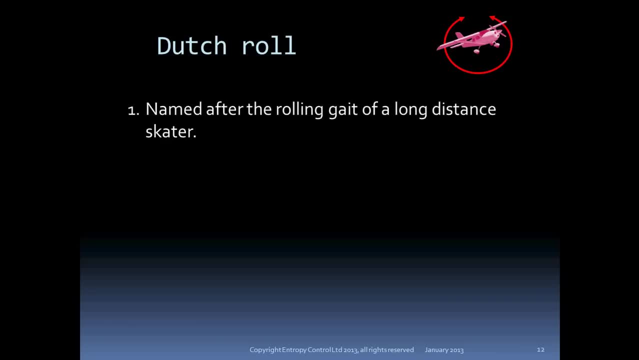 Dutch Roll is caused by too much stability and sideslip. It's a rolling and turning oscillation reminiscent of the motion of a long-distance skater and roughly the same period. In Dutch Roll, the aircraft snakes around the sky. The aircraft yaws and rolls to the side, a movement that eventually self-corrects. 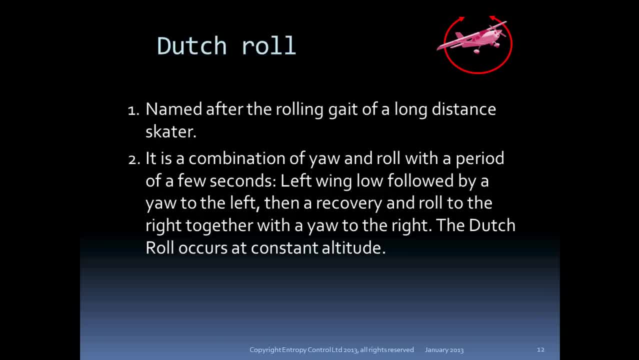 but goes past the straightened level into a yaw and roll on the other side. This happens more or less at constant altitude. The period is in the order of a few seconds, but the motion is remarkably difficult to control. Dutch Roll is usually in a trade-off with spiral stability. 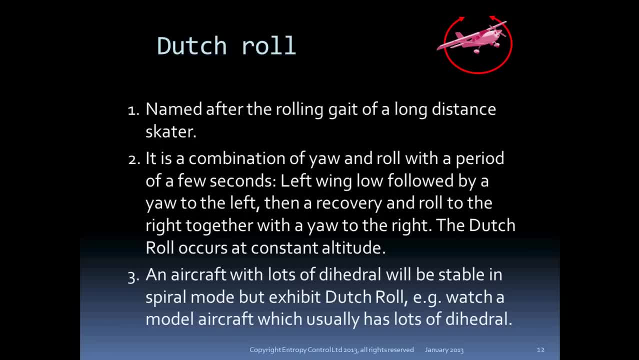 Model aircraft, for which the seconding motion of Dutch Roll is not a problem, usually have much more dihedral than passenger aircraft. This gives good spiral stability, but you'll often notice the wings on a free-flight model continuously rocking, which is their very nature. 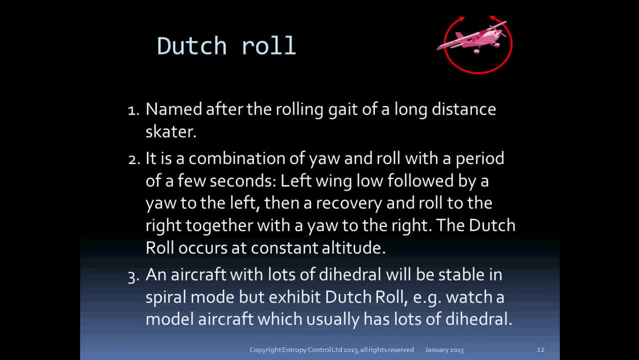 This is their version of Dutch Roll. Dutch Roll will make you and your passengers sick very quickly, which is why it tends to be eliminated at the cost of loss of spiral stability. Large aircraft that are not rigid and can flex significantly often have their own subsets of Dutch Roll occurring in the tail. 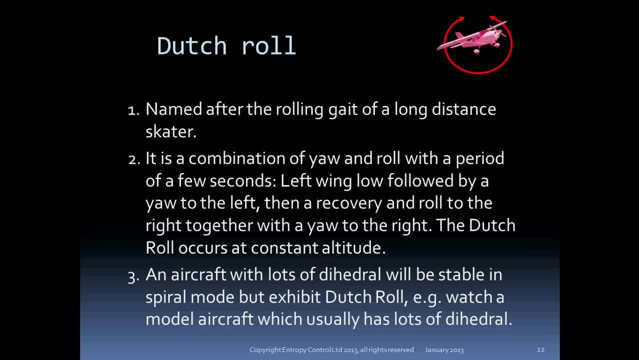 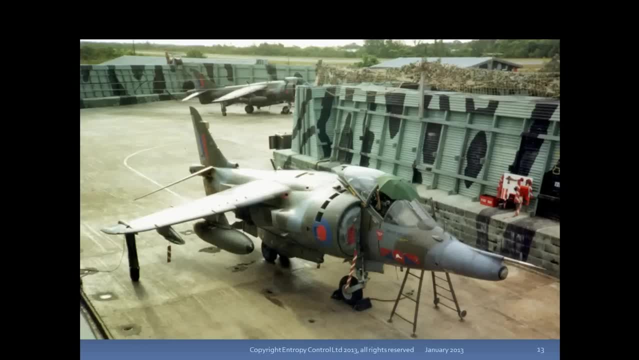 The Boeing 747 suffered from a weaving in the tail section that was eventually cured by an automatic yaw damper. This is because of the dihedral sweepback and high wing position. all enhance sideslip stability, but is possible to have too much of a good thing as far as sideslip stability is concerned. 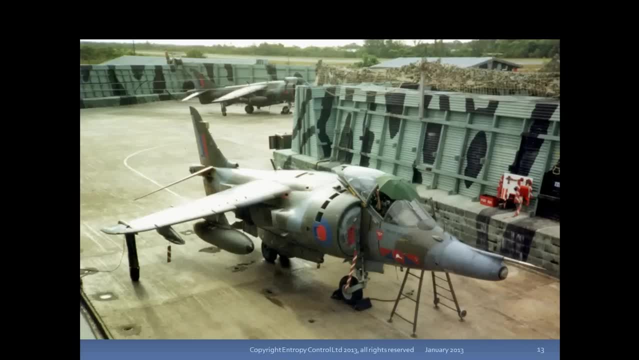 Too much introduces Dutch Roll instability. So you'll see normally that high-wing swept-wing aircraft will also have marked anhedral or negative dihedral to reduce sideslip stability. You can see that here in the Harrier aircraft. Note that the tailplane also has anhedral to help reduce sideslip stability. 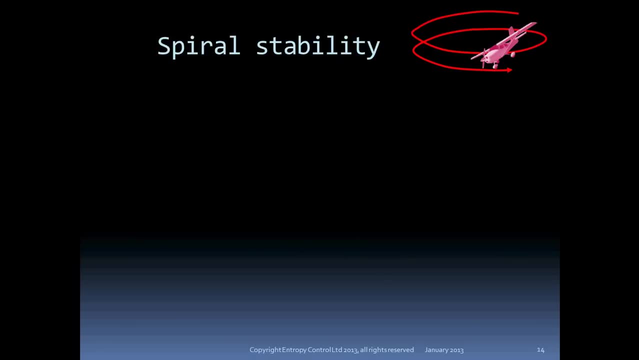 Now, if you don't want Dutch Roll, then often your only choice is to accept some spiral instability, and that's what happens in practice. So most light aircraft have no spiral stability. Try releasing light aircraft. Try releasing the stick in level flight and giving the rudder a kick. 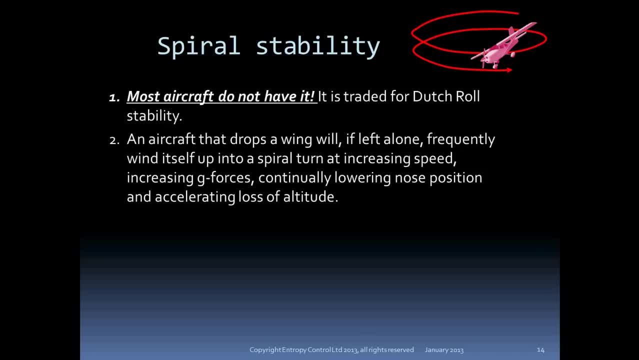 After the aircraft rapidly returns to forward flight because of its short-term yaw stability, there will be a gentle, balanced turn that, if left on its own, steepens and tightens with constantly increasing speed as the nose drops. This process is very gradual in the beginning. 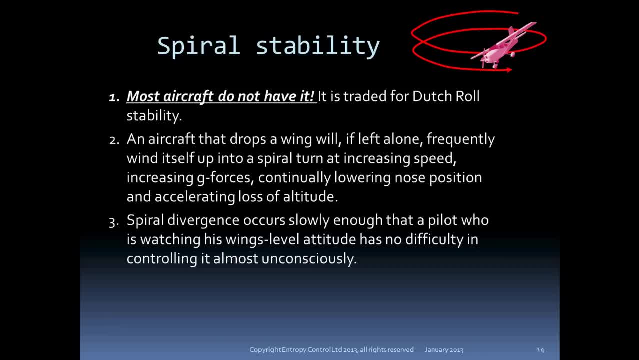 so a pilot with a good horizontal reference corrects almost unconsciously for it at all times. But this is what causes the famous graveyard spiral that can occur when VFR pilots lose the horizon. in IMC conditions, The spiral tightens and speed increases as the aircraft heads down.